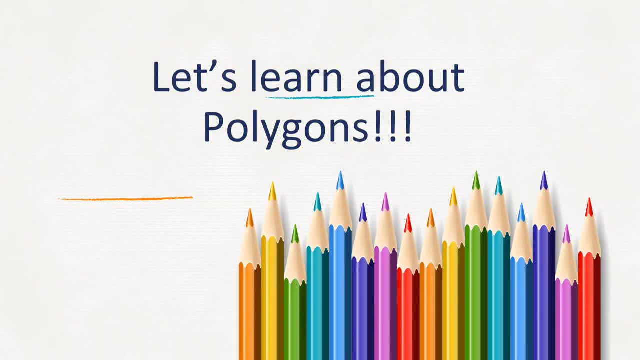 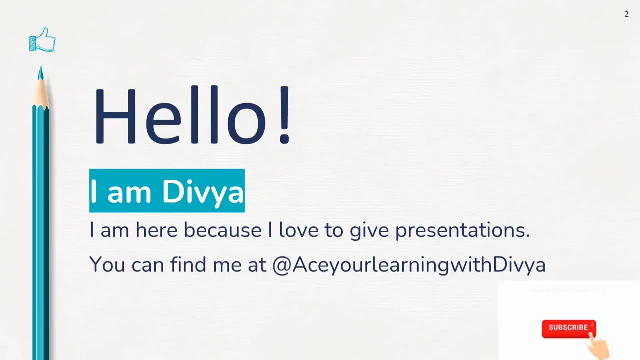 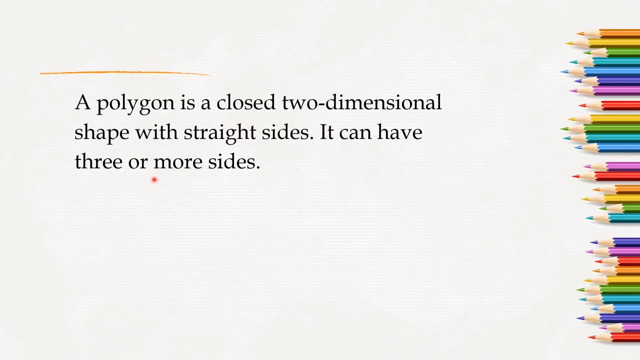 Hello, welcome back to our channel, Asia Learning, with Divya Students. in today's video, let us learn about polygons. What is polygon? A polygon is a close, two-dimensional shape with straight sides. It can have three or more sides. Look at this figure. 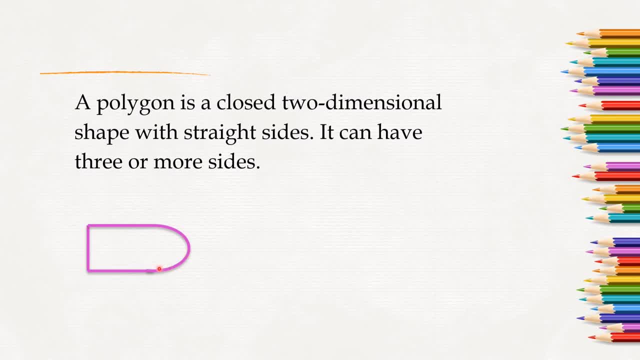 Is it a polygon? No, it has a curved side. It is not a polygon. Look at this figure. Even though this is a closed figure, it is not polygon because it does not have straight sides. Look at this figure. Is it a polygon? Yes, it has straight sides. Also, it is a closed figure. So this is a polygon. 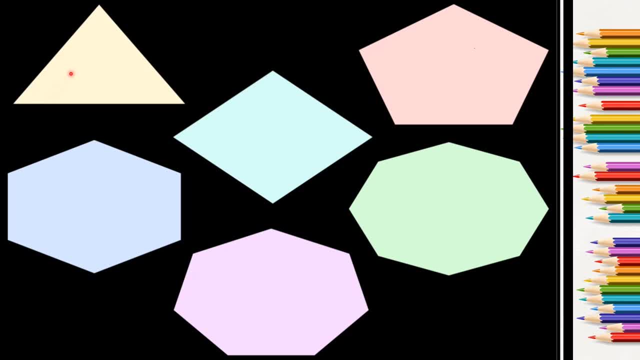 So polygon is a closed figure, form, line segment and not curves. Yes, and it is two-dimensional figure. Poly means many and gone means sides, So the shapes which will be having many sides are called as polygons. It can be triangle, it can be square, it can be rectangle, it can be pentagon, it can be octagon, it can be. 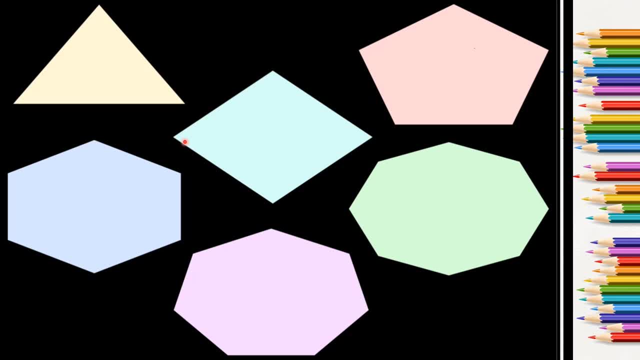 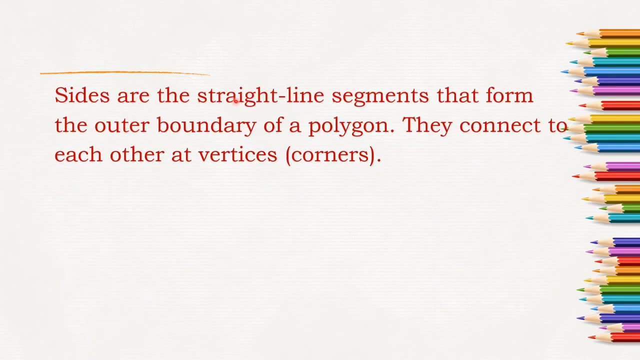 hexagon. It can have n number of sides, but it has to be a closed figure and should not have curves. Next, what are sides? Sides are the straight line segments that form the outer boundary of a polygon. They connect to each other at vertices. Vertices means corners Here. 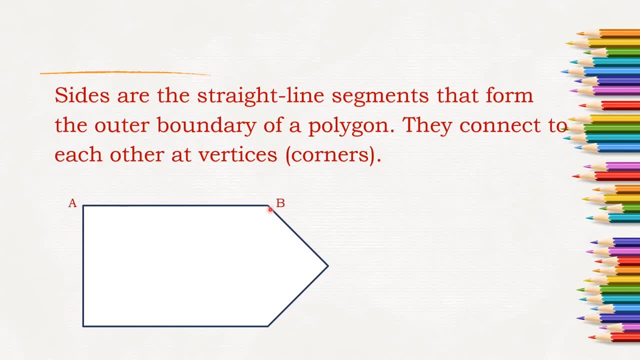 A, B, C, D, E, F, G, D is a line segment and it is a side Right. Also, B, C is a line segment and it is a side of the polygon C. D is a line segment and it is the side of the given polygon D. E is a line segment and 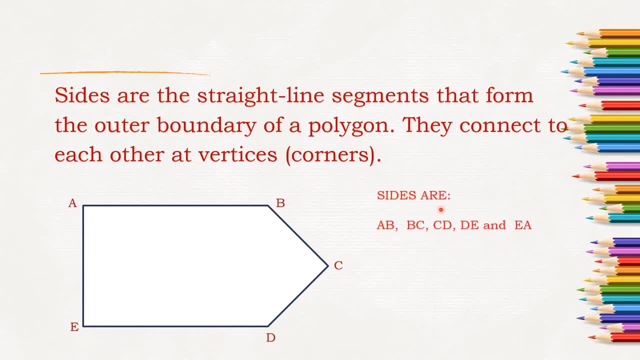 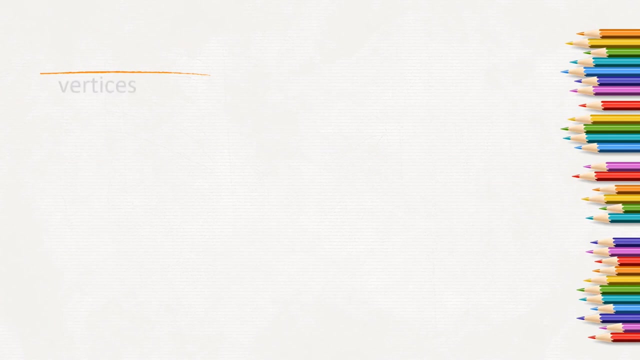 it is a side of a polygon. Here the sides are line segment A B, line segment B C, line segment C D, line segment D E and line segment E A are the sides of the given polygon. Next, vertices, Vertices, are nothing but the corners where two sides meet at a common point. 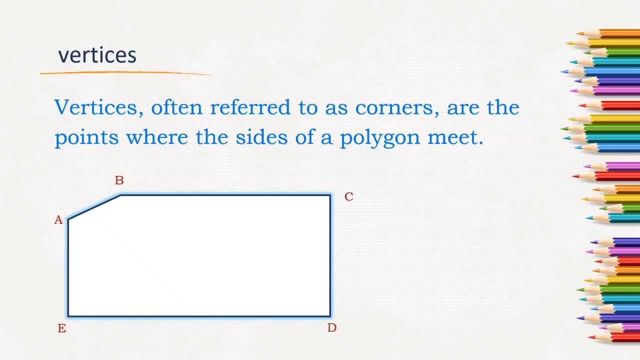 is called as corner Right. So here, line segment A, B and A, E are meeting at a common point, A point of A and A, B and D, C are meeting at a point of D, B and C, D are meeting. 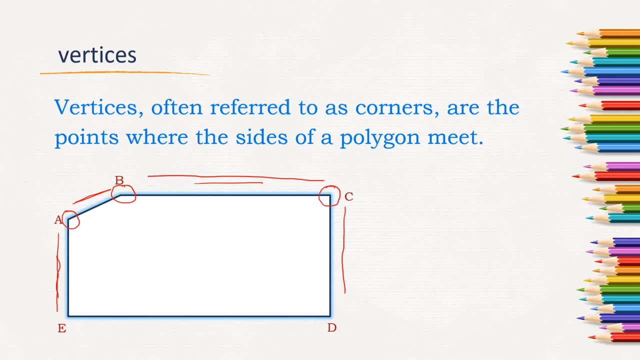 at a point of C and C, D and E. D are meeting at a point of D, D, E and T and A. E are meeting point of E. So here the vertices are the meeting points A, B, C, D and E Vertices. 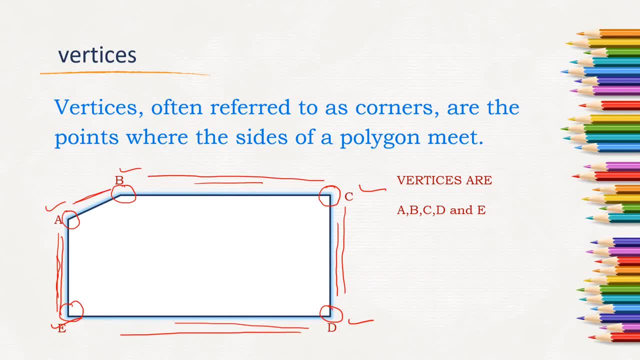 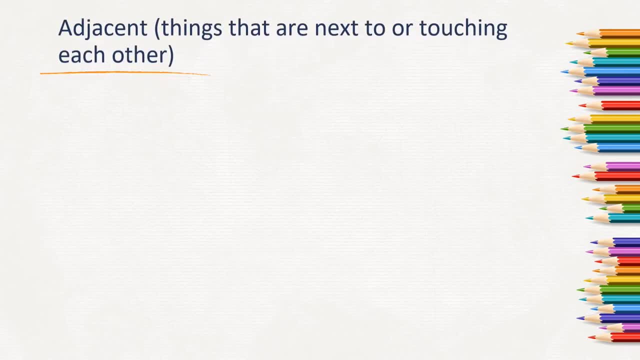 of a given figure are A, B, C, D and E Adjacent. Adjacent means things that are next to each other or touching each other Right. So here in polygons adjacent sides are sides that share a common vertex, that is corner. In the figure A, B line, segment A, B is adjacent to B, C, A, B. 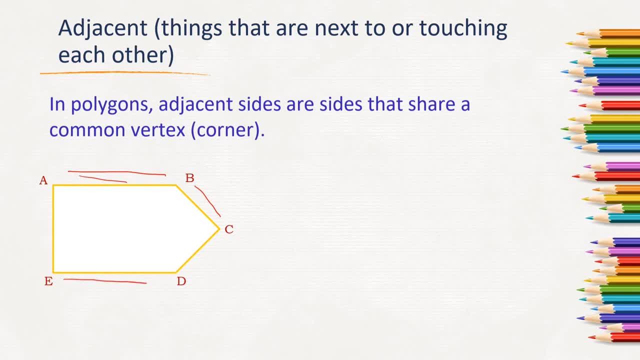 can't be adjacent to E, D, Right, Because they are not touching each other. They are not next to each other, Right? So here in polygons, adjacent sides are sides that share a common vertex, that is corner. So A, B will be adjacent of B, C and B, C will be adjacent of C, D, D, E will be adjacent. 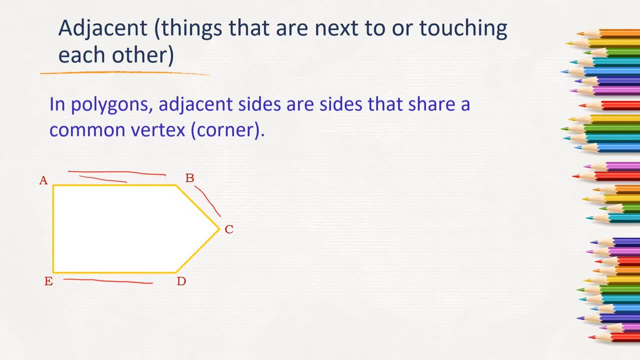 of A- E. When they meet at a common point, then only they are called as adjacent sides. Here line segment A, B and line segment B- C are next to each other and they are meeting at a point. So these line segment A, B and line segment. 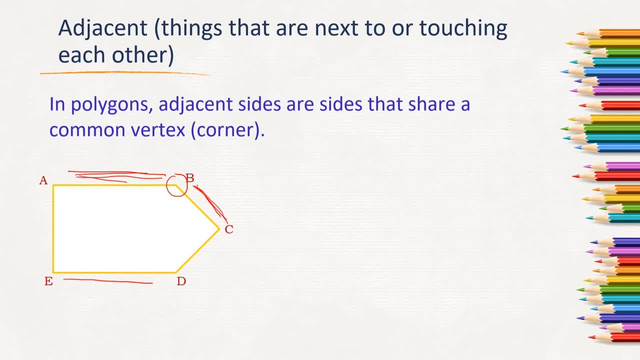 B- C are adjacent sides. Similarly, B, C and C- D are meeting at a point and they are next to each other. So line segment B, C and C- D are adjacent sides. So here A B, line segment A, B and. 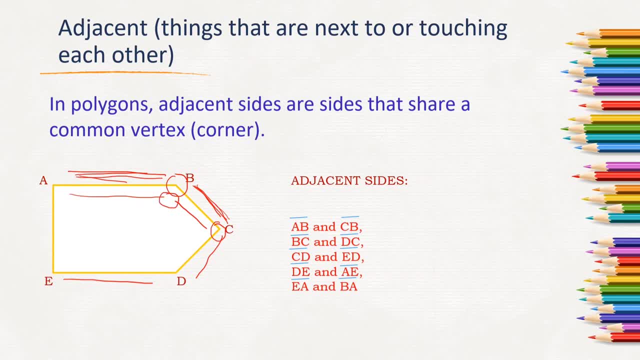 line segment C- B. both are meeting at a point, So line segment A, B and C- B are adjacent sides. Similarly B, C and D- C are adjacent sides. C, D and E- D are adjacent sides and D, E and A- E are. 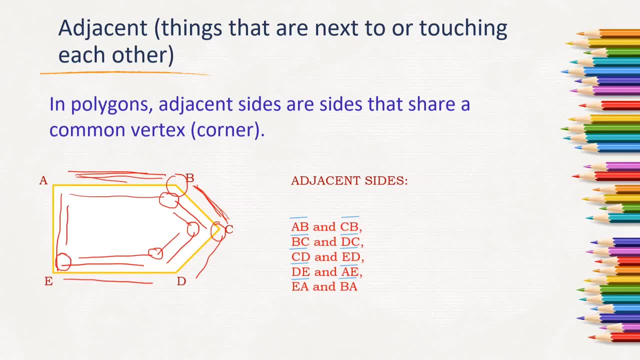 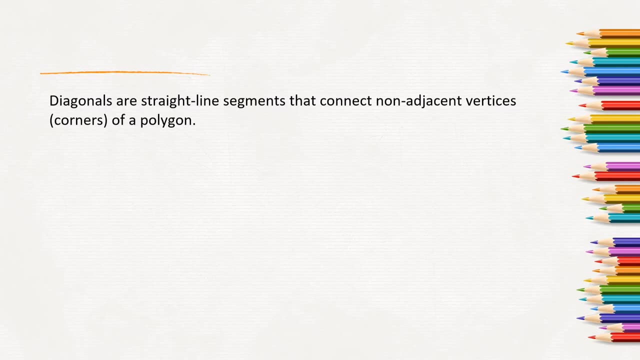 adjacent sides. E A and D A are adjacent sides. So line segment A, B and C- B are adjacent sides. Diagonals: What are diagonals? Yes, diagonals are the straight line segments that connect. non-adjacent vertices means not next to each other. vertices means corners of a polygon, The. 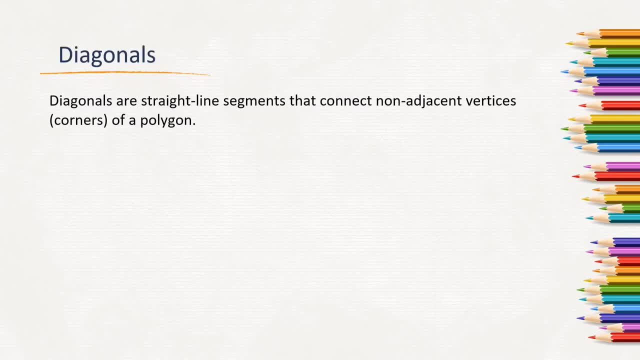 corners should not be next to each other. So when we connect to the vertices which are not next to each other it becomes a diagonal. So here is a figure. So we have to join any two vertices which are not joined by any side. So here A, B are sharing a common side, So we can't 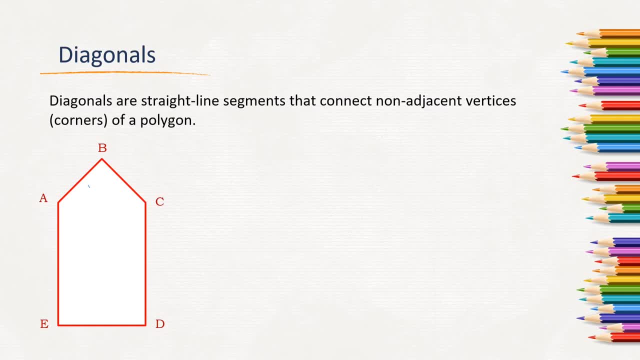 mark a line segment here. We can't mark a diagonal. here We can from A to C. Here the vertices are not next to each other, right, And the sides are also not next to each other. A, C and then A D, and then can we connect with A, E? No, 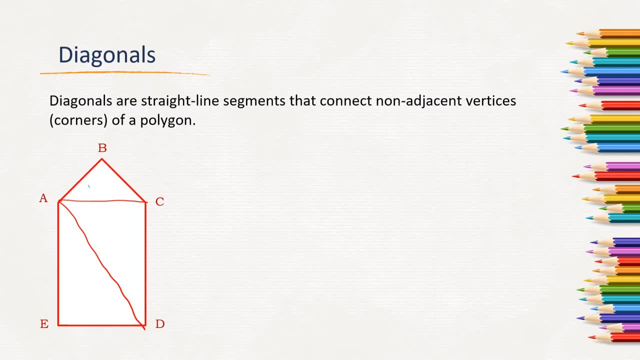 No, No, Because they are sharing a common side. Next, moving to B: B cannot be connected with A or C, right, Because they share a common side. So next we will be connecting to D and then to E, as they are not sharing a common side. Next, moving to C: C cannot be connected with. 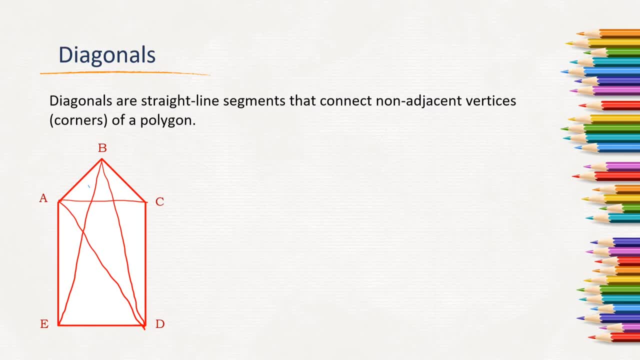 A, which we have already done, and can be connected with E also, So we will connect with E also. Moving to D: D cannot be connected with C or E, So it can be with B and A, which is already done. 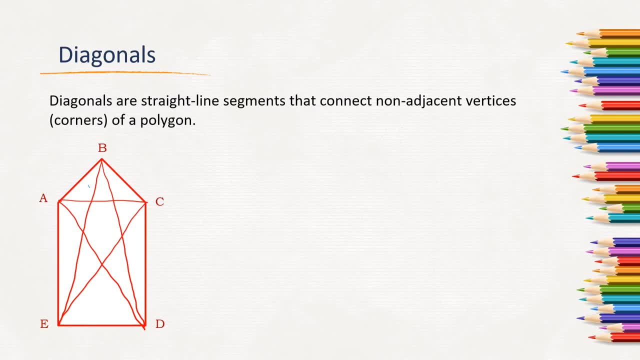 Similarly, E cannot be connected with A or D, but can be connected with B and C, which is already done. So here are the diagonals: Line segment A- C, Line segment A- D, Line segment B, D, Line segment B, E, Line segment C, E and D, A, which is: 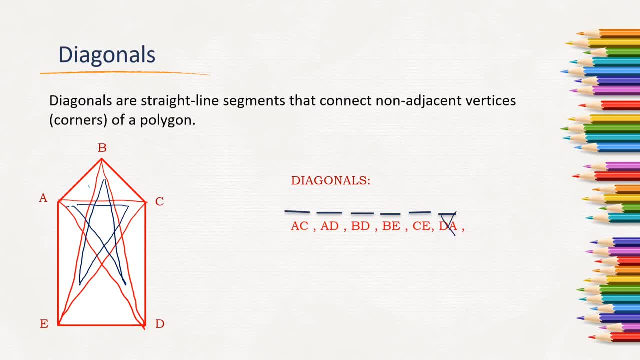 already done, So five diagonals, which is all. D, A is already done, So here we will get five diagonals, that is, A C Line segment. A C Line, segment, A D Line. 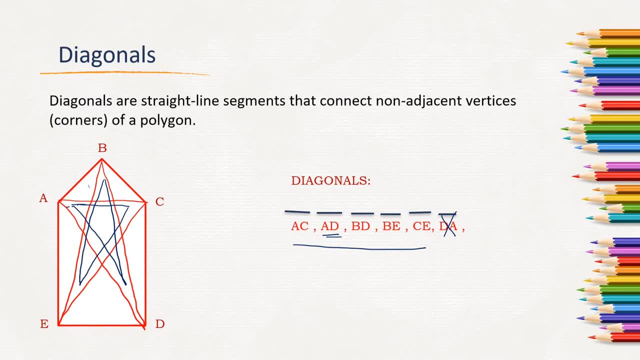 segment B D, Line segment B E and line segment C E are the diagonals for the given polygon. Now look at this figure. Can we find a diagonal for a triangle? No, because all the vertices share the sides. 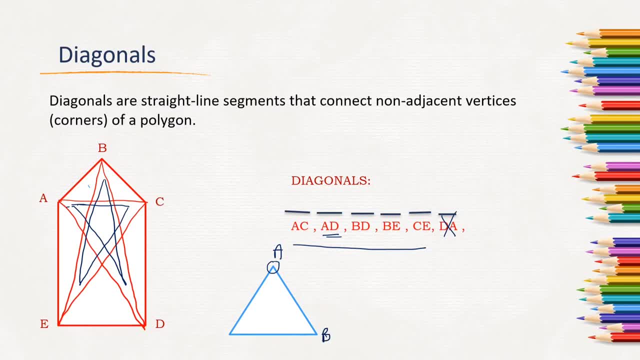 For example, this is A, B and C. For A: C is also connected. D is also connected right, And for B, C is connected. A is also connected. For C also, B is connected and D is connected.